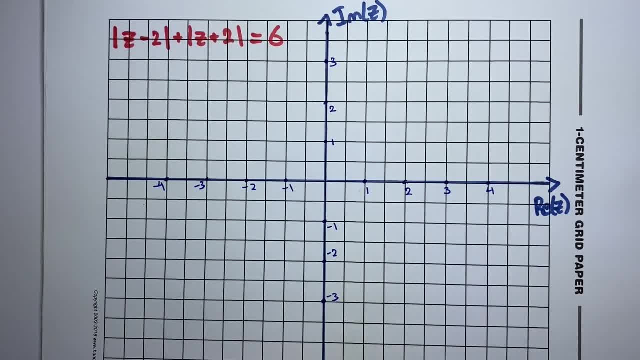 video right now. have a go at trying to actually express what this is saying in words. So the way that I would describe it is, I would say something along the lines of: it's the set of all complex numbers, z, such that it's: 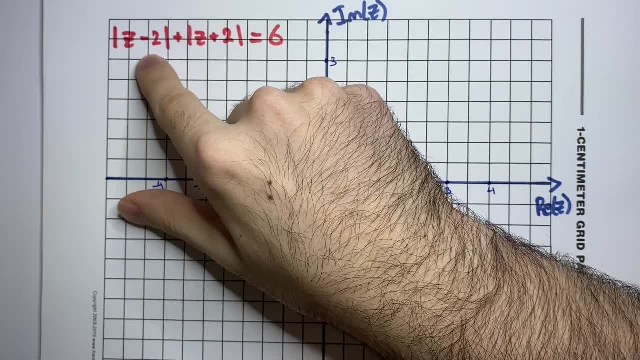 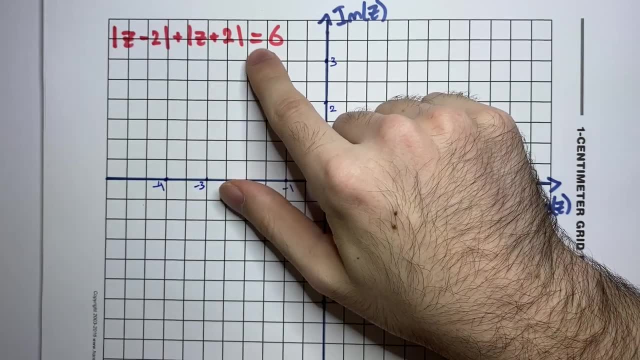 distance from the complex number 2, which is represented by this bit, plus its distance from the complex number negative 2, which is represented by that bit. there It's equal to a constant, and in this case our constant is 6, and we'll see. 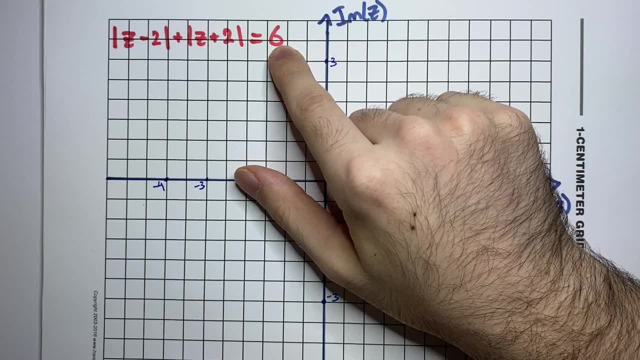 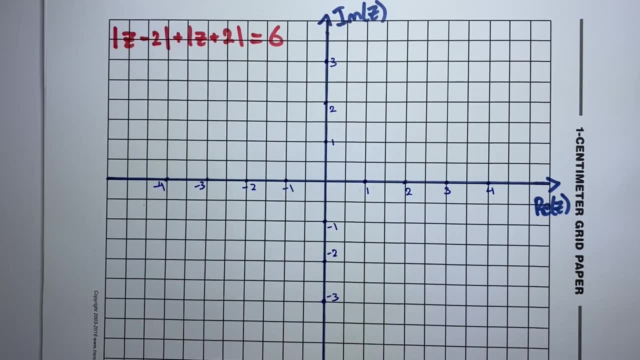 later on that this is actually quite an important value in order to understand what our curve looks like. Alright, so that's the way that's how I would describe it. Maybe you have a different way of describing it, but hopefully it's along the same lines. Now, what we want to do is we want to get a piece of string. 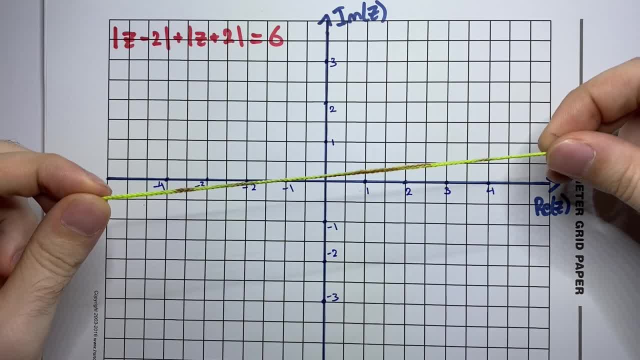 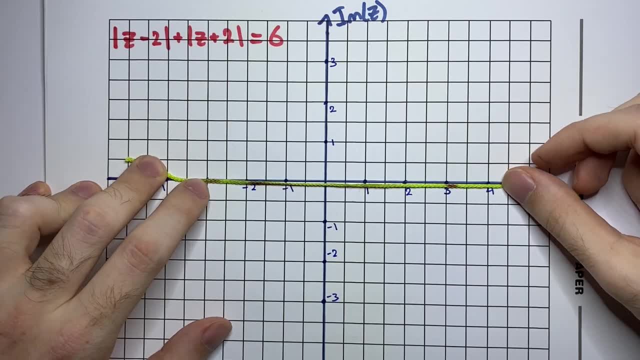 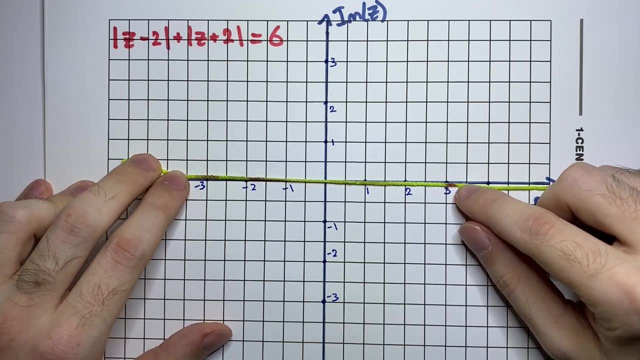 and we want to mark off six units. So, oh, it's a little bit hard for you to see, but I've actually. you might be able to see that there's a bit of a red texture here on the point negative three and a bit of red texture on the point positive three. so that's now mapped out. 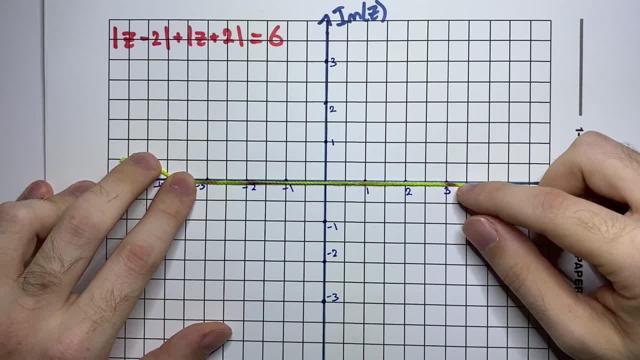 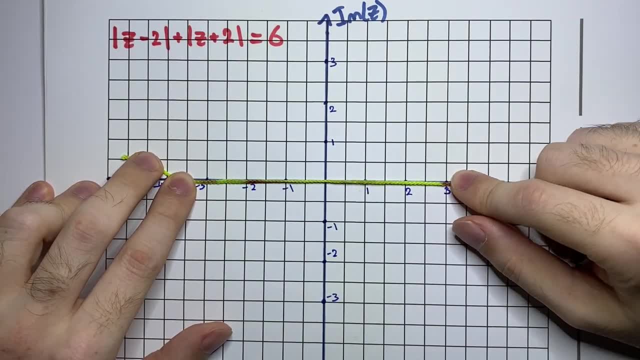 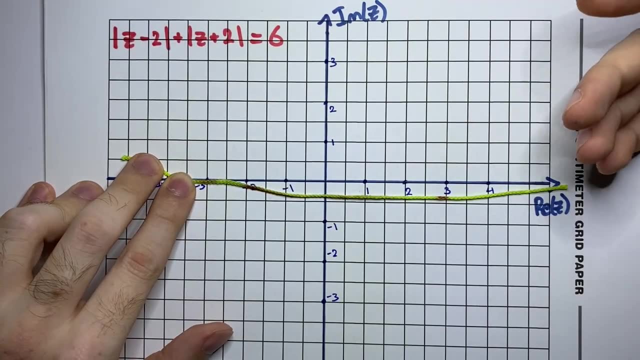 or marked out six units, Okay, and what we want to do is we want to to use this string to help us form our curve. Now let's go back to what the locus is. The locus says that it's all the points z, and remember, z is a variable point. Now 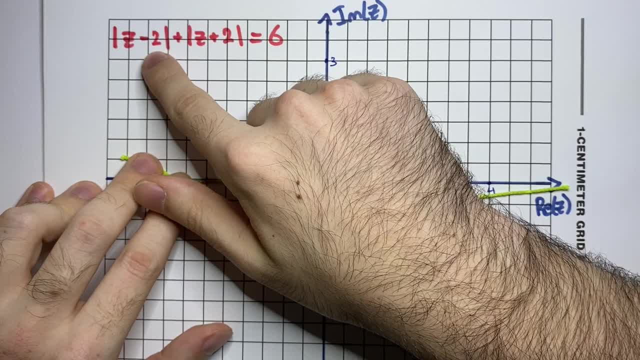 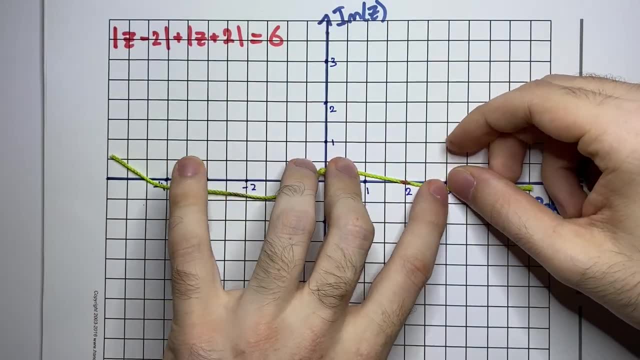 It's all those points z whose distance from 2 plus their distance from negative 2 is equal to 6.. So we want to lock these points in where we marked. We want to lock those in at 2 and negative 2.. And to do that we're going to use a thumbtack. 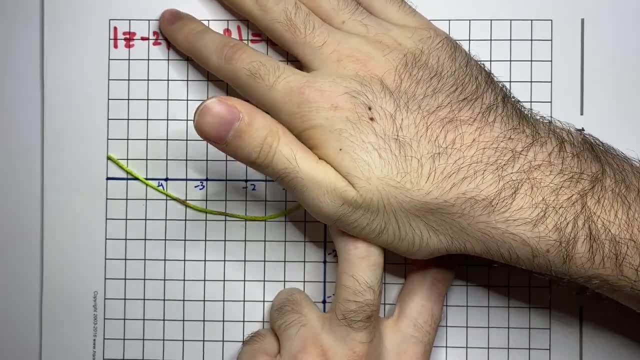 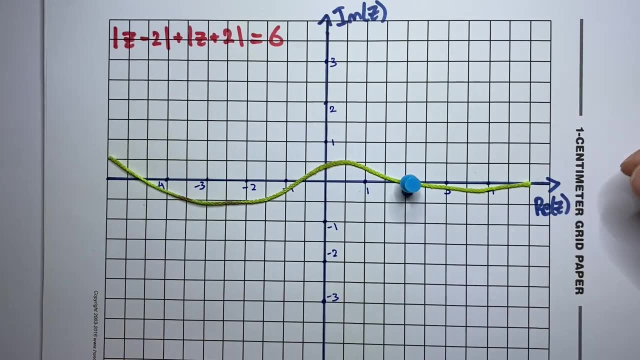 Now what you'll need is you'll need to make sure that underneath your grid paper you have some old paper, or maybe an old exercise book, so that you can actually stab it in. It doesn't go into the table and wreck the table. 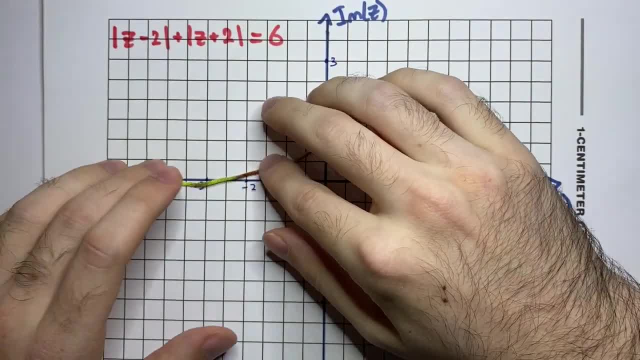 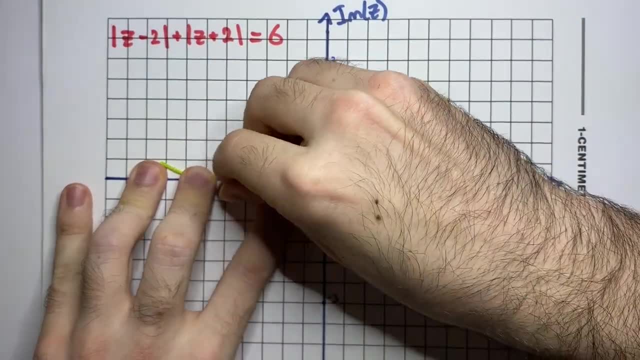 Okay, so we've locked one in at the point 2.. Let's do the same at negative 2.. Let's get the other thumbtack. put it in at negative 2. And again, make sure you push down very hard. 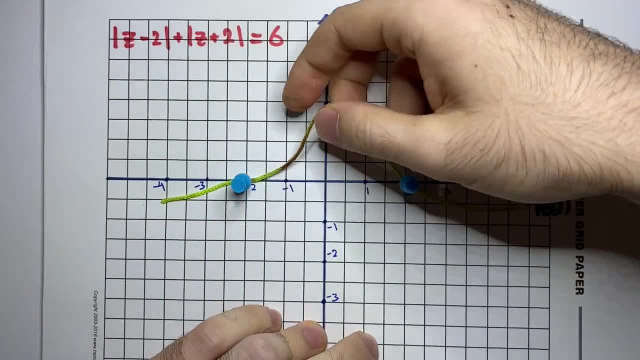 Cool. So now we've locked that in at 2 and negative 2.. And the distance between these two points along this string should be 6, because that's what we marked out. So now we've locked that in at 2 and negative 2.. 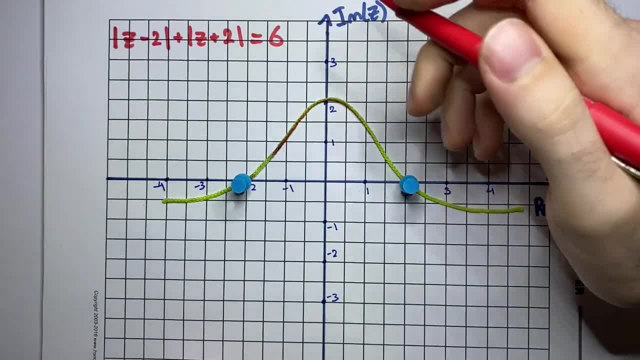 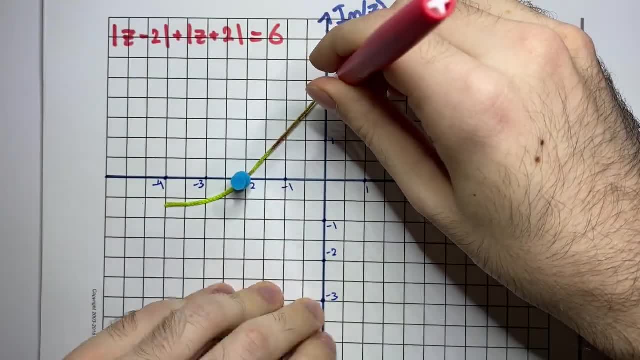 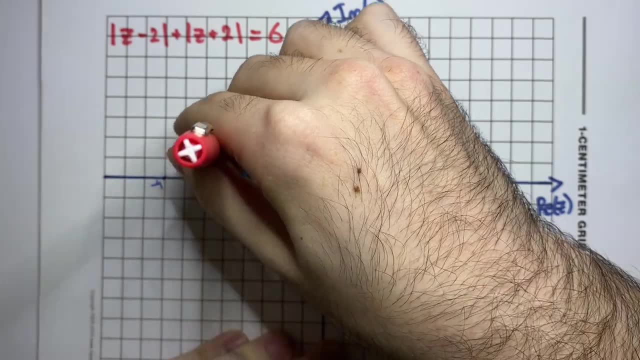 So now we get our pen- and I would suggest getting a different colored pen to the axes- And we make sure that our string is actually tight, because otherwise it's not going to work, And we draw out our locus. So what's happening now? my pen is the point Z. 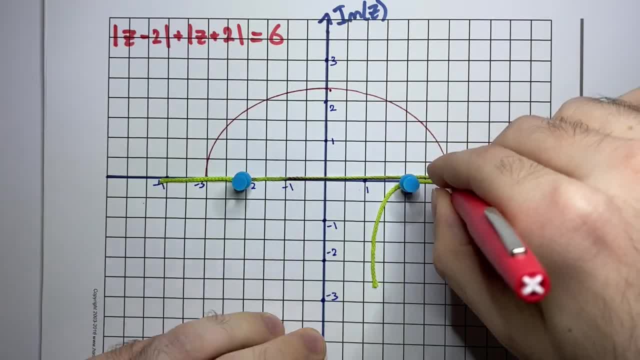 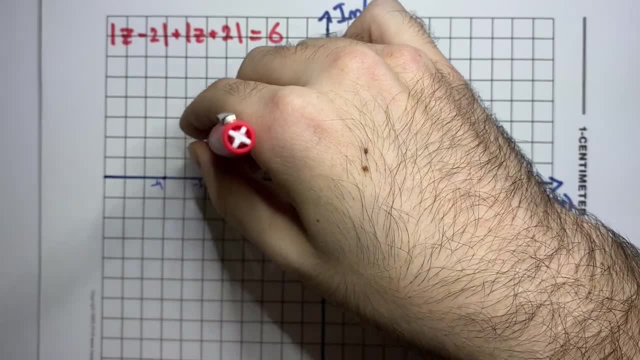 and it's being constrained such that its distance from negative 2 plus its distance from 2 is always equal to 6.. Okay, remember, 6 is the length of our line, of our string. Okay, and you might be able to see what's going on. 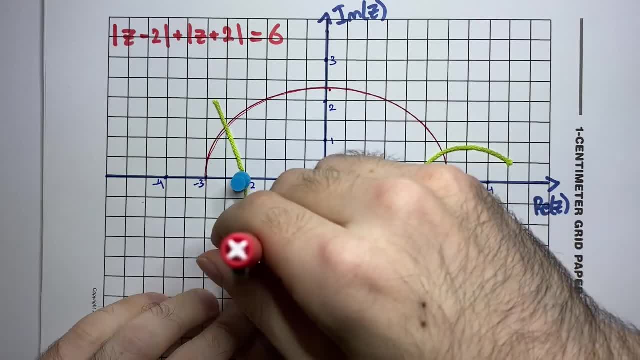 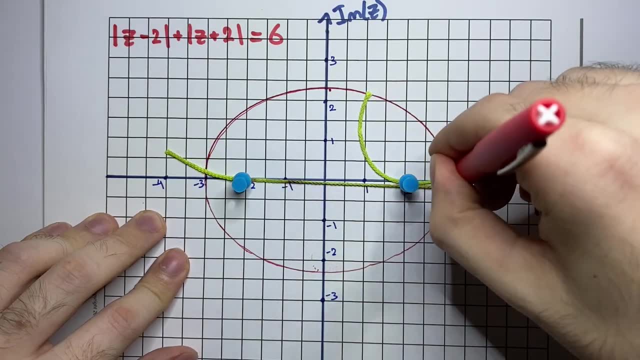 Let's do the bottom as well, But we're going to get a very nice. it's like the pen's screwing up a little bit, but we're going to get this very nice curve which is known as an ellipse. Now let's take that off. 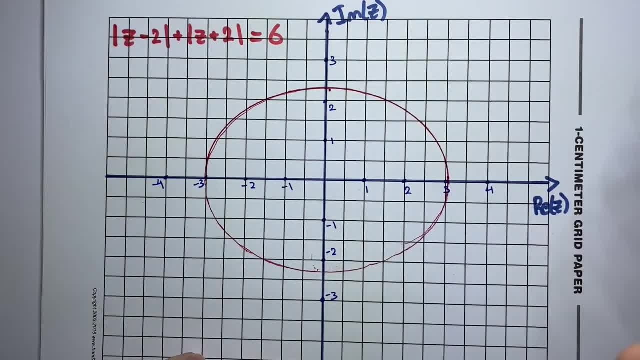 So there you go, we get our ellipse. Now the study of ellipses is no longer in the extension 2 course, unfortunately, or fortunately, depending on how you look at it. It was part of an old topic called conics, but that has now been taken out. 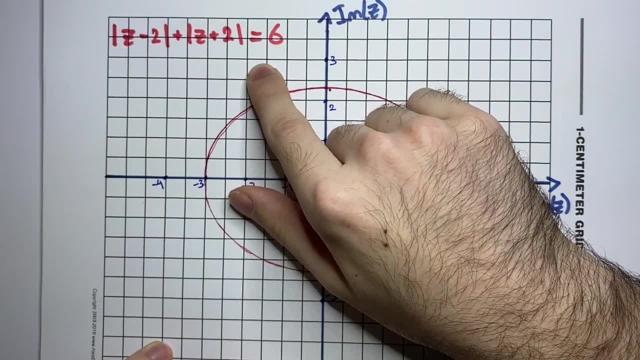 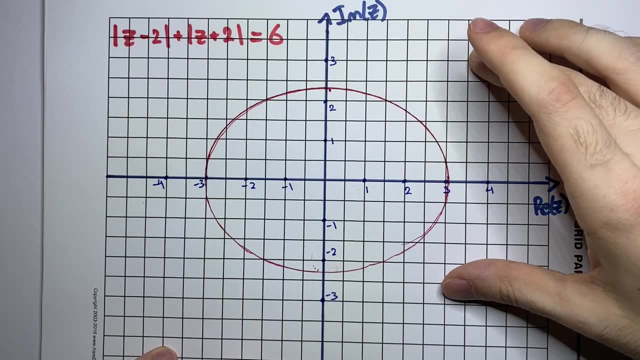 However, there are still some textbooks which have this locus form in there as part of the complex numbers, locus or regions in the complex plane. So that's why I thought it's a very important example to go through in detail, because you get a bit of an understanding of why this shape. 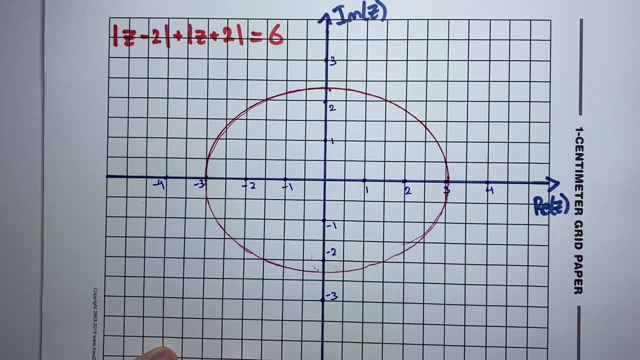 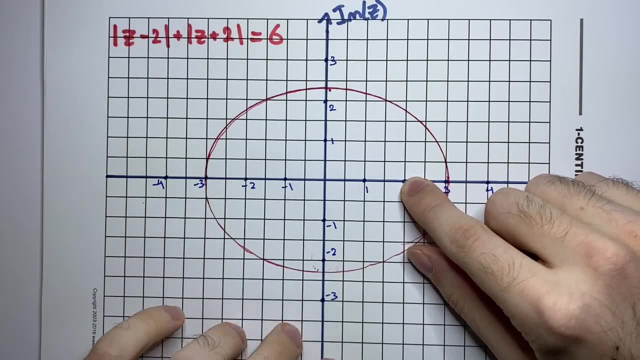 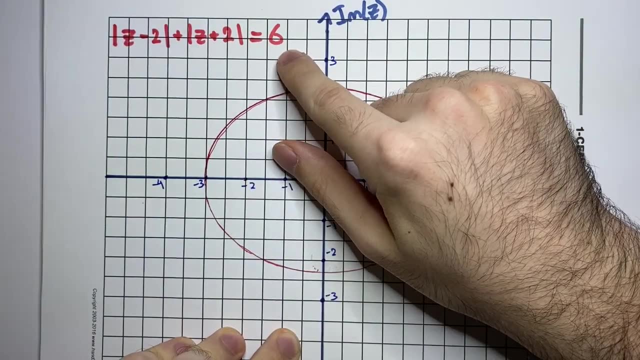 or why this form actually forms this shape known as an ellipse. So one of the ways of defining an ellipse is that it's the point or it's the curve whose distance from two points is always equal to a fixed constant. Now we said that this point 6, or this number 6, was really important. 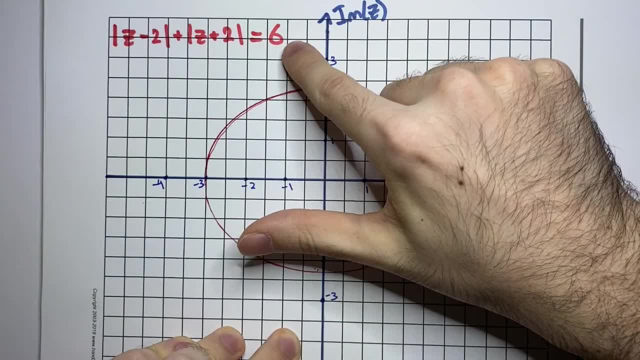 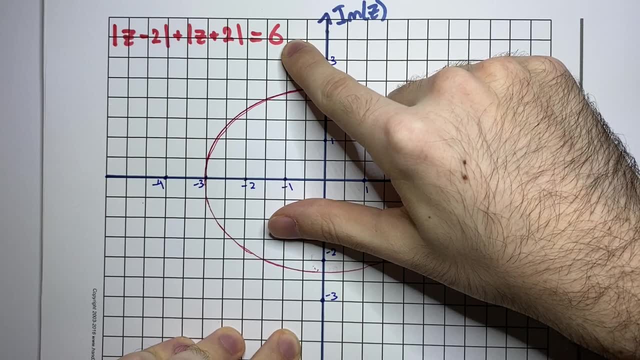 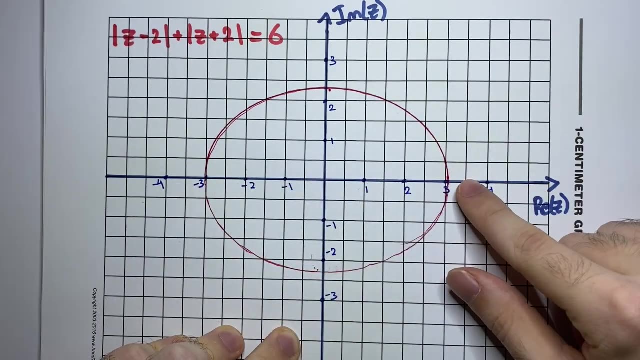 Now, what's important about it? Well, 6 is actually twice the major, the semi-major axis, or you can think of it as the length of the major axis. Now, what is the major axis? Well, the major axis is the length of the longest axis. 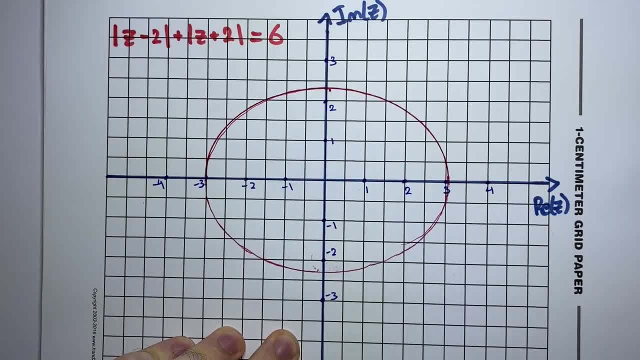 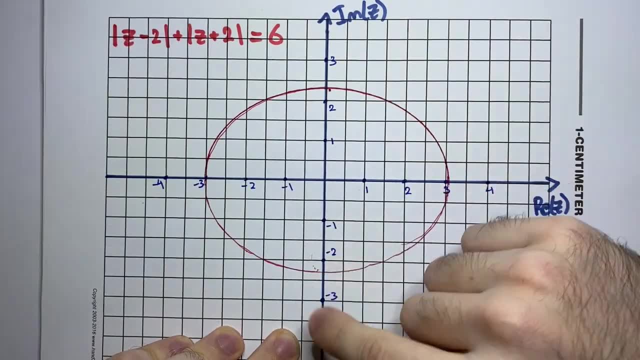 So in this case, that looks like it's the horizontal axis here. Okay, so this is known as the major axis of our ellipse, All right, and the smaller one, well, that would be known as the minor axis. But yeah, this point 6 is very important, or the value 6,. 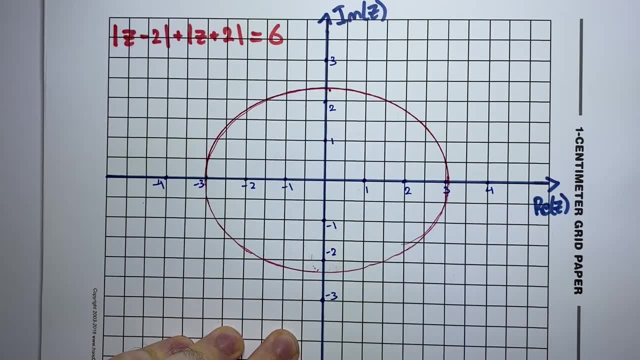 because it tells us what our major axis of our ellipse is going to be. Now, what I would suggest for you to do is to think about what happens when we change the value of 6.. If we kept everything else the same, what happens when we change that value 6?? 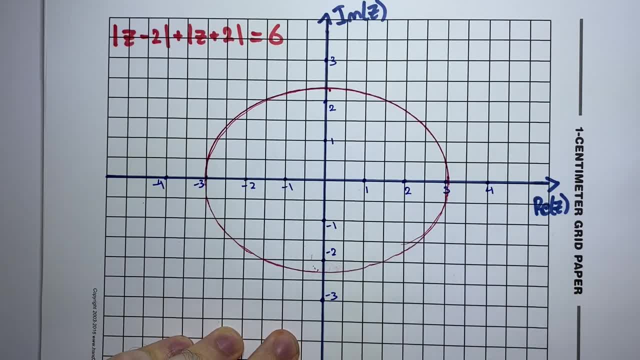 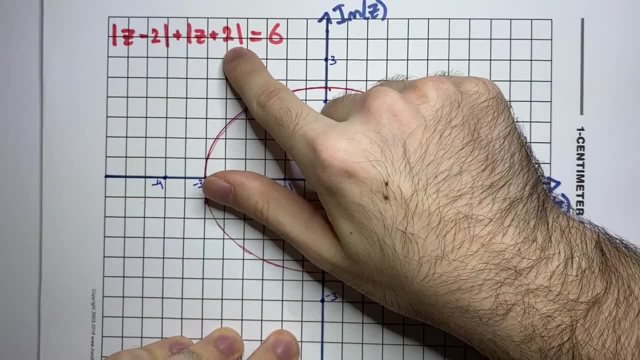 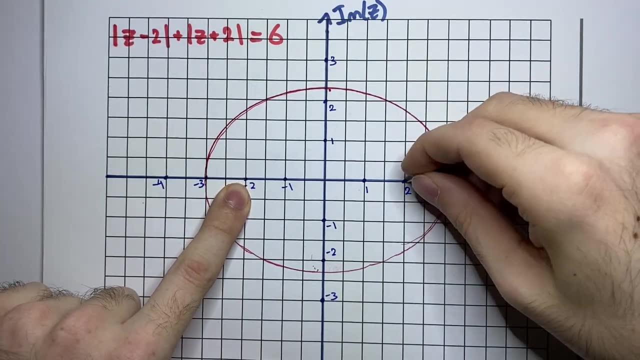 Are there any values that wouldn't work? Are there, or what values would work? Maybe you can think about that. And then these two points 2 and negative 2, so those were where we plugged in, or plugged in where we stabbed in our thumbtack. 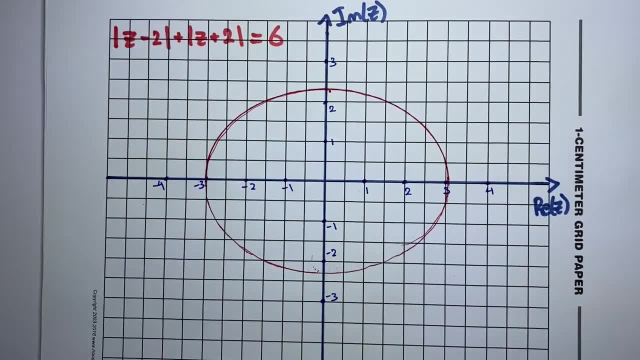 These are known as the foci of the ellipse. Now, when you're graphing this ellipse, something that you really should do is you should definitely mark out your foci. Okay, so you really want to mark out this point here and this point here. 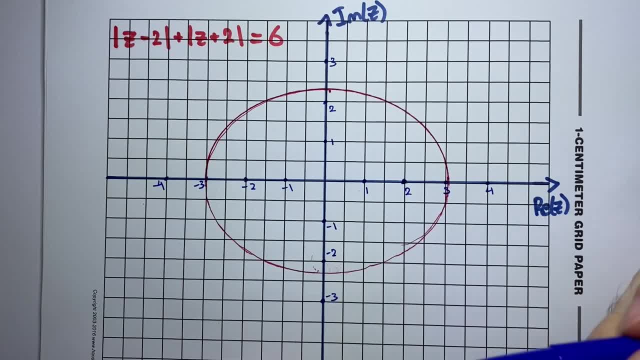 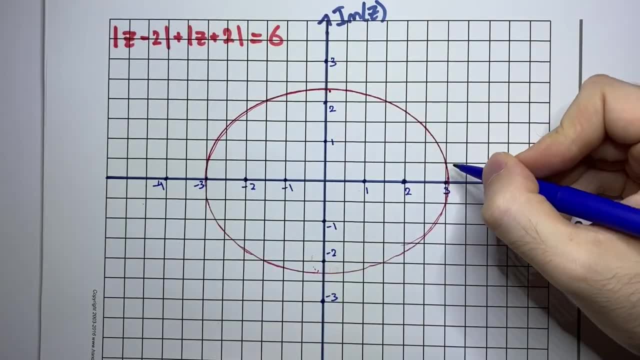 because these are our two foci. It's also really good to mark out your intercepts. So in this case we've got the intercept. here is 3.. Now, I can see that it's not exactly on 3 here, but that's because the texter 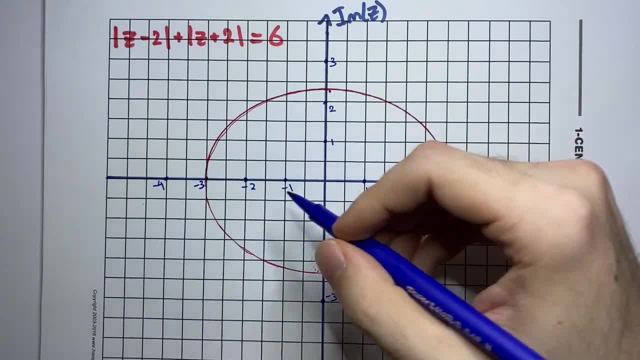 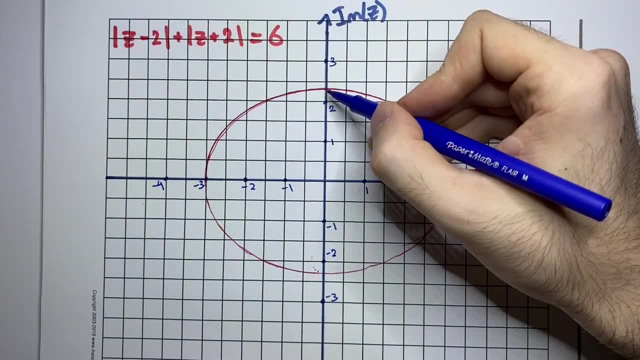 has a thickness, the string has a thickness, but we know that this is going to be 3, because we know that the whole thing should be 6, and our center is at 0.. Okay, so this, definitely, we know that this is 3, but how do we work out this point? 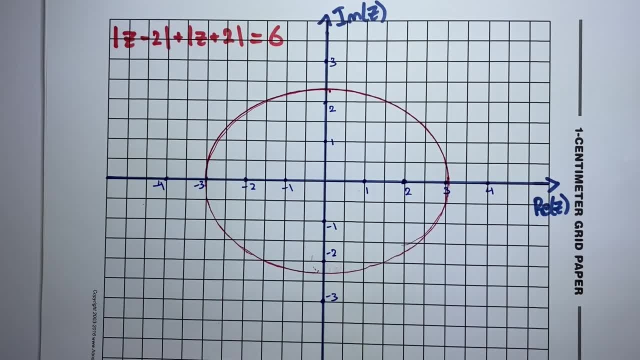 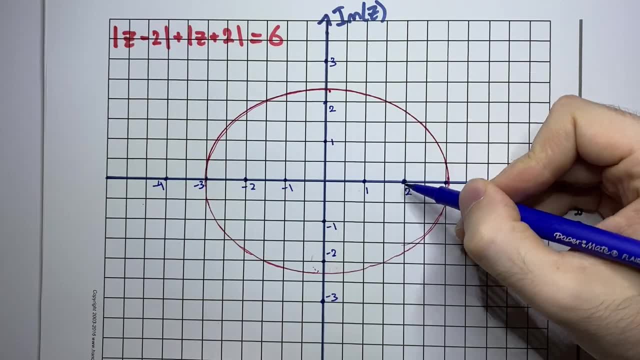 Well, that's a good question, A good way of thinking about this. what was the constraint? The constraint was that the distance from negative 2 to 2 should always be 6. So that should apply at any point on our curve here. 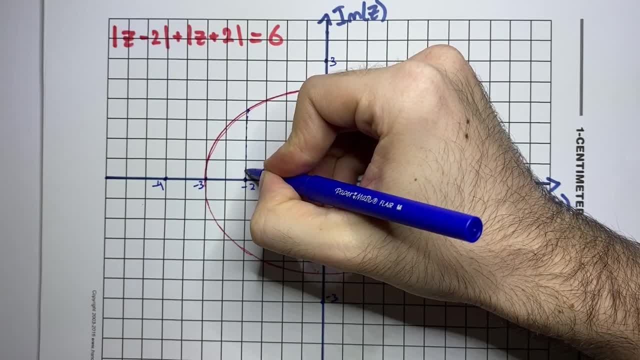 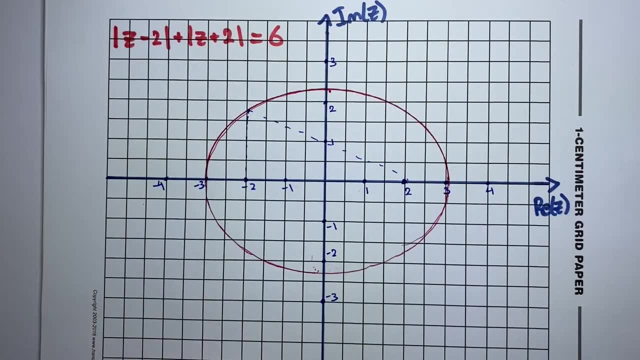 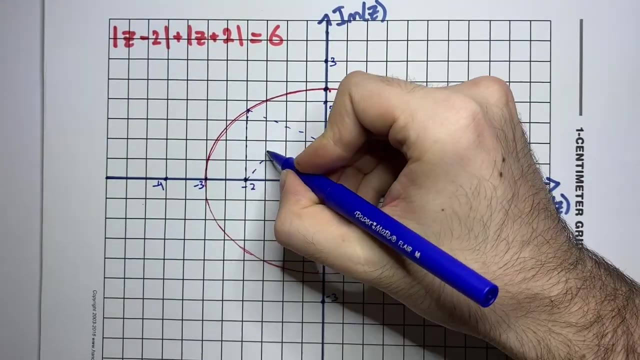 So that means that this point here and then this distance- if we added them all up, that should be 6.. So why can't we just have a look at this point here? It's a very particular point, but it's going to do a world of wonders for us.